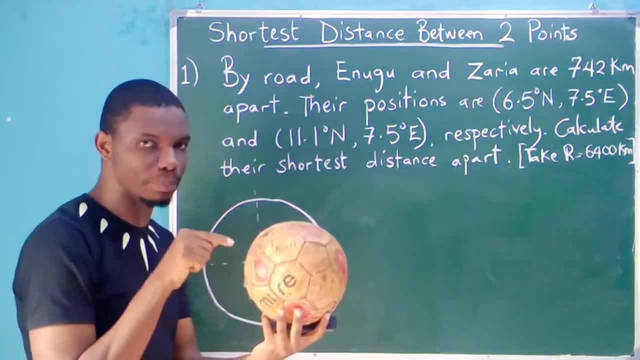 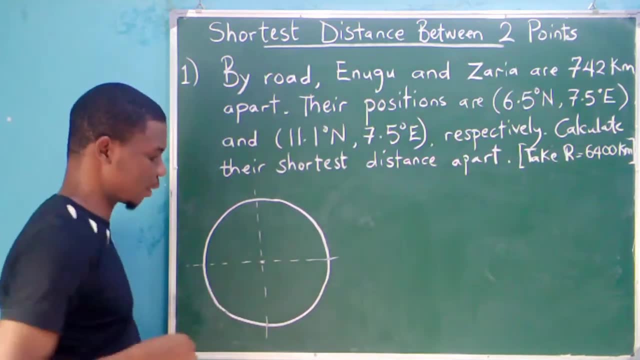 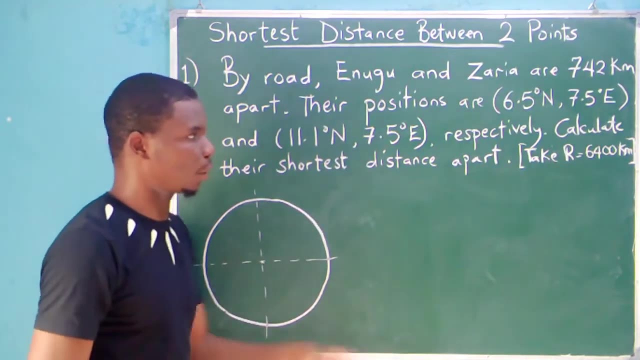 and this other one going from here and coming out from here where they meet at the center. that will be this part here, Okay, so that you understand what that center is, what I'm talking about. All right, Now. the next thing is to locate the points that you are giving For any point on. 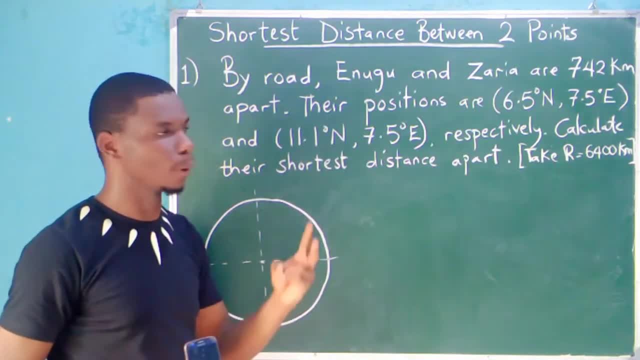 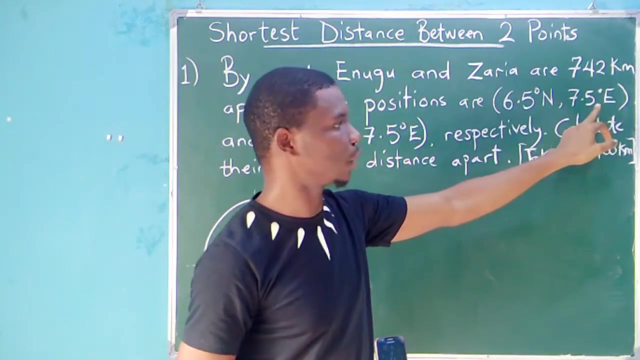 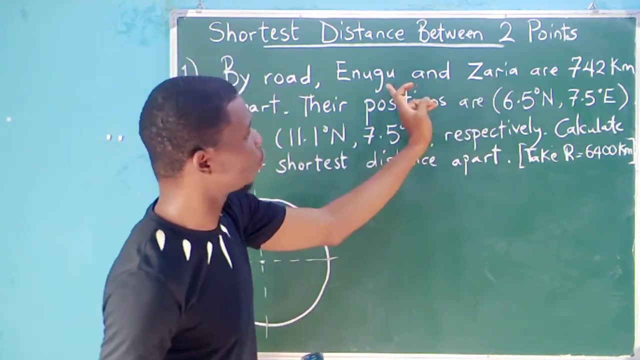 the earth's surface, we can use two markers to indicate it, two coordinates: the longitude and the latitude. okay, and when we are giving these points, we are first giving the latitude before the longitude, the latitude always before the longitude. okay, so for this one, for zari, for enugu. 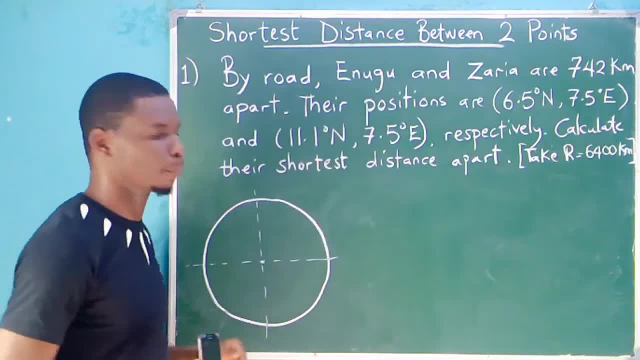 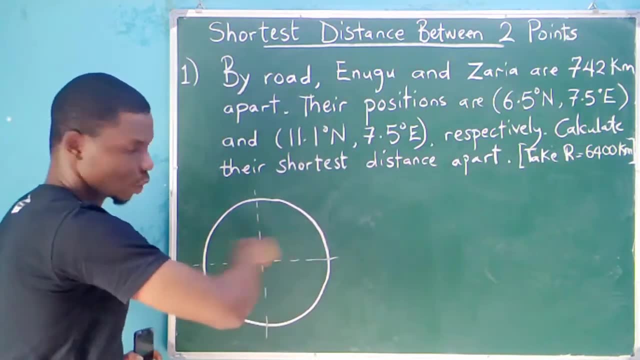 enugu is 6.5 degrees north. now, where is north? the long latitude, are the ones that go like this or the ones that go this way? you know, horizontally, like this, they are the latitude and north is from this line upwards is north, and then down from this line downwards. 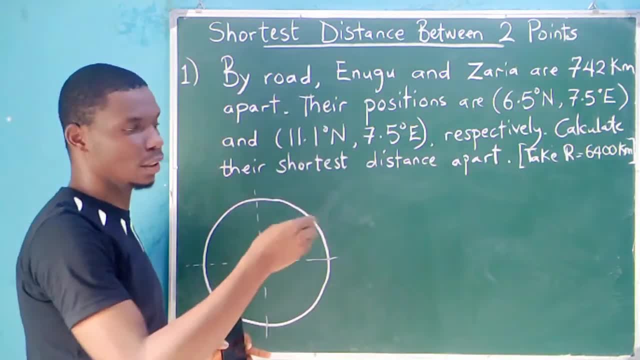 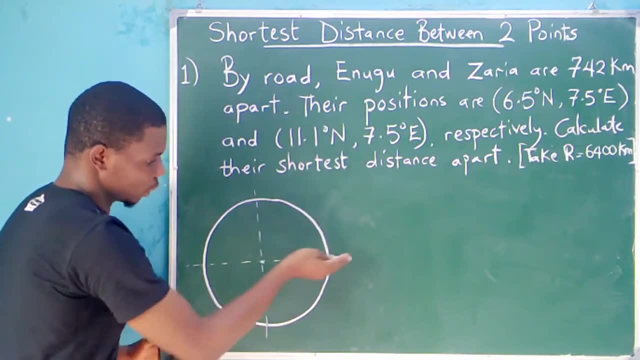 is south. so it means that 6.5 degrees north will be above this line, above this line. so it goes from this line. this line is the zero degrees. it goes from this line up to 90 degrees. so we can mark our 6.5. let's just say: this is our 6.5. okay, that's 6.5 degrees north and then 7.5 degrees. 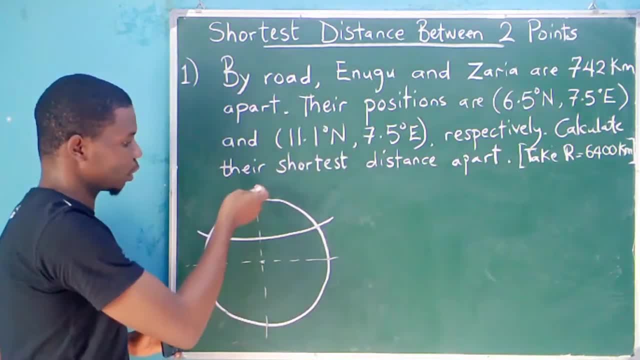 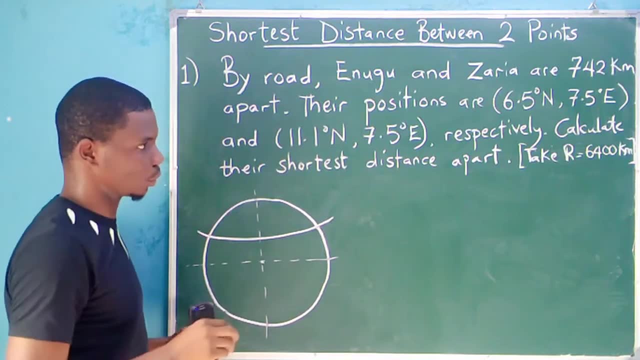 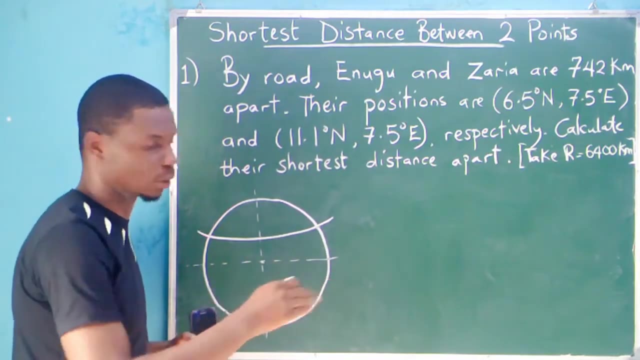 east. now for latitude, latitude, longitude are the ones that go from up down. you know, all these ones that go from up down, they are the longitude. and this side, your right hand side, is the east direction, while your left hand side is the west direction. so, from this line to this side, east from this line, this way is west. 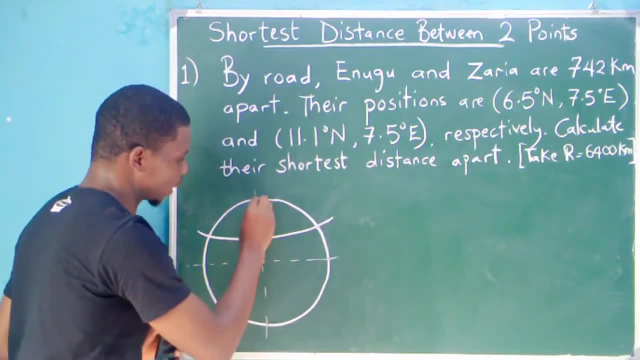 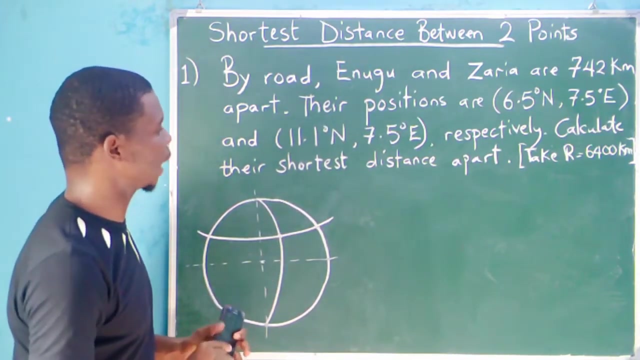 so 7.5 degrees east. so we are going to mark it like so. okay, all right, so we have indicated this first point. so this will be where enugu will be. this point here where they meet, then for zarya, zarya is 11.1 degrees knots. 11.1 degrees knots it means it is above this one. this one is: 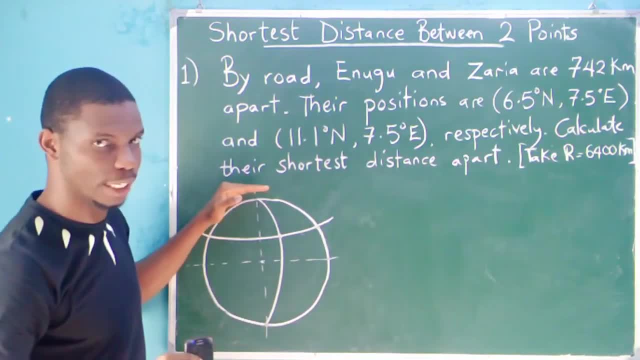 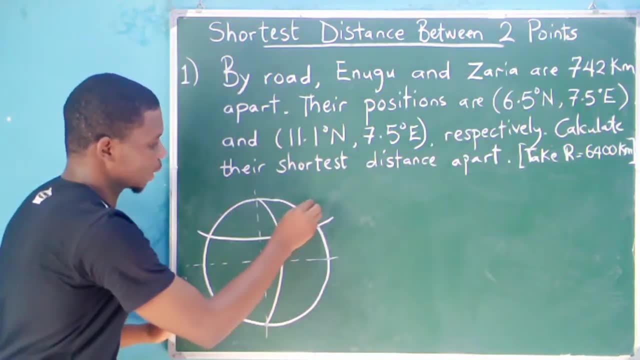 6.5 and we are going from 0 to 90, right. so it means 11 will be on top of 6.5. so i can mark it like this. now, these markings are not exact. you don't need to make it exact, i'm just trying to make it, you know. 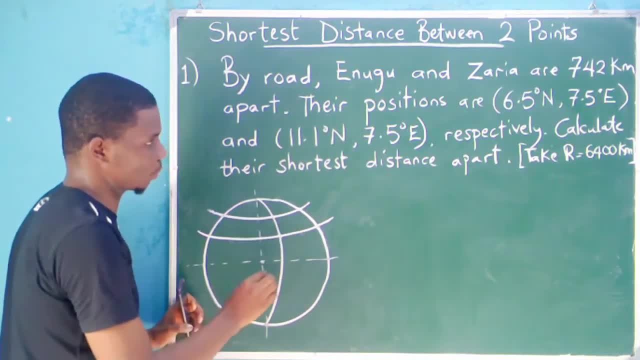 give space so that you can mark it like this, and then you will be able to mark it like this, so you you understand it will be visible. If not, I would have drawn them close together Like 6.5 and 11.5. needs to be a little bit close together. 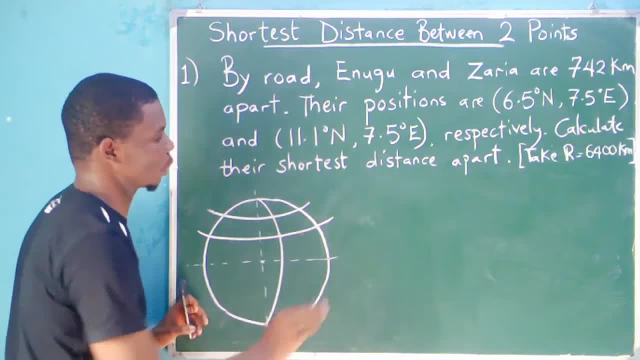 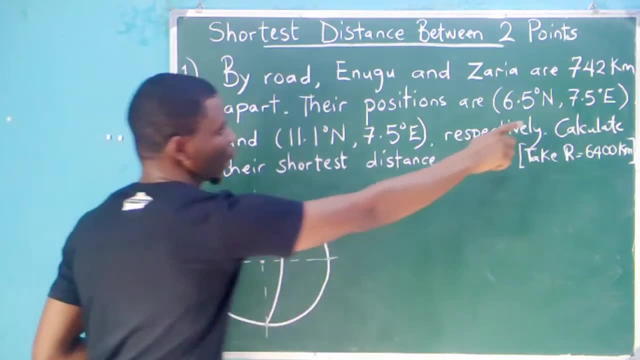 But I'm giving this space so that there will be space for us to see what we are drawing. Then, 7.5 degrees east is the same thing with this other one: 7.5 degrees east. 7.5 degrees east. 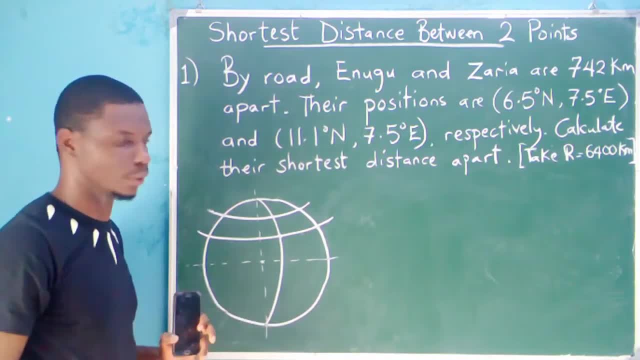 So both of them are on the same longitude. okay, So this will be our Zarya. So this is Zarya, and then this is Enugu, And remember that this is the center of our Earth. Okay, now we want to calculate the shortest distance apart. 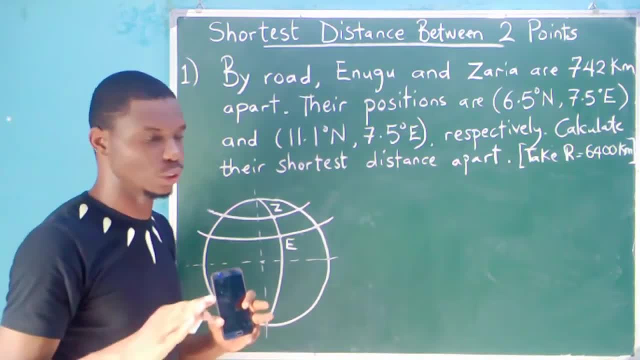 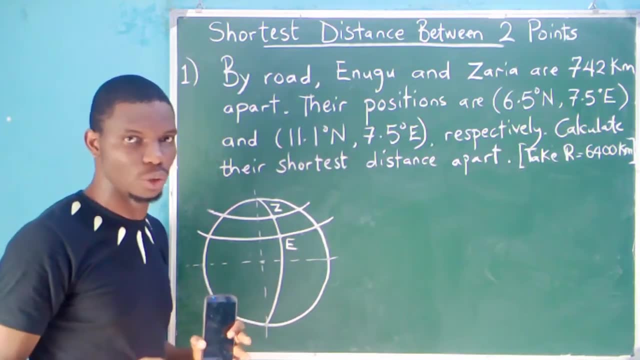 Now, anytime you're asked to calculate the shortest distance between two points, it is usually the distance along a grid cycle. And what is a grid cycle? A grid cycle is any cycle on the Earth that has a radius of the Earth. Okay, so like these ones, all these lines of longitude. 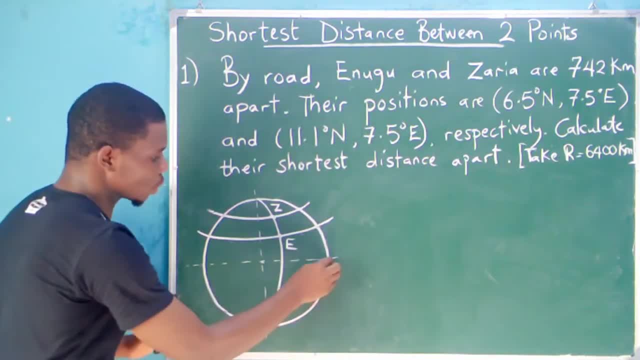 all of them have the radius of the Earth, But the ones latitude. okay, you can see this one and this one, they don't have the same radius. This one is bigger than this one, Now, the only one that has the radius of the Earth. 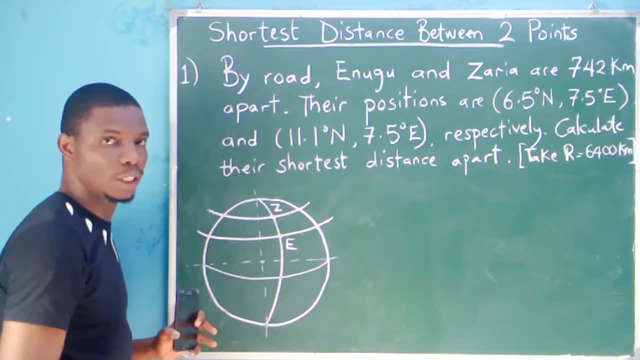 is this one at the center which is the equator. That is for latitude But for longitude. all the lines of longitude are grid cycles, So it means we are looking. we are looking for the distance between Zarya and Enugu along this grid cycle. 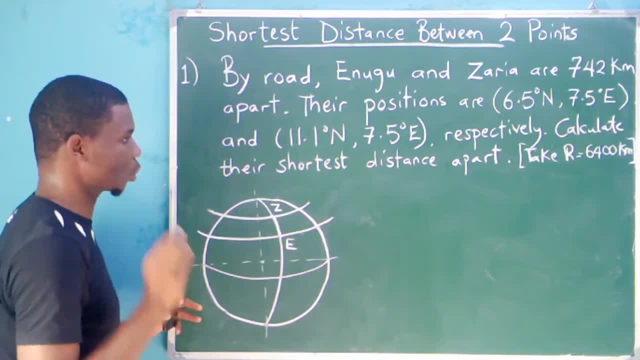 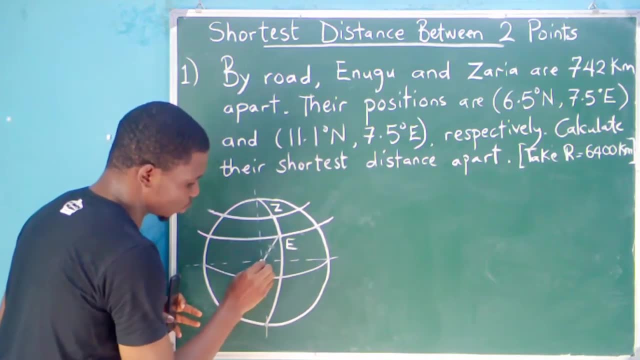 So this is the distance we are looking for. Okay, that will be the shortest distance between the two points. Now, from the center of the Earth. I can draw, I can just draw the radius. Okay, so this will be like the radius. 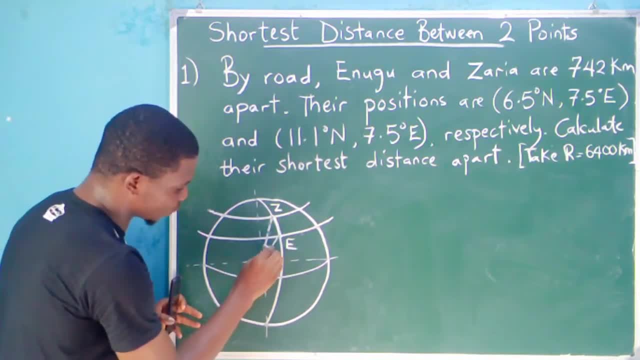 Now, from here you can see we have formed an arc. Okay, We have formed an arc. This is the radius of the Earth. this one, This one also is the radius of the Earth. So we have formed something like an arc this way. 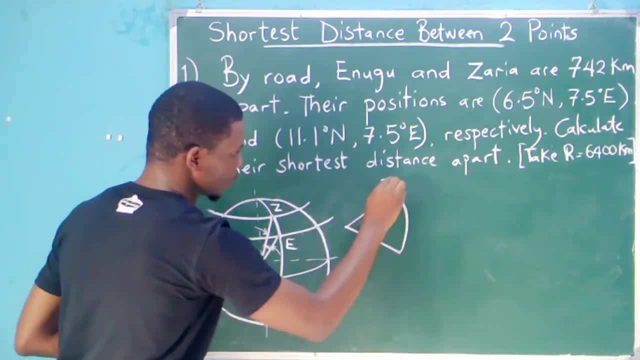 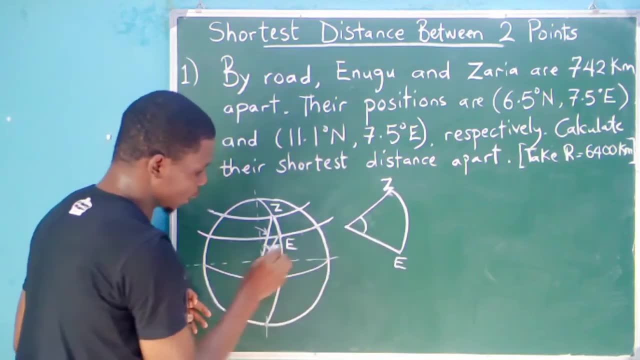 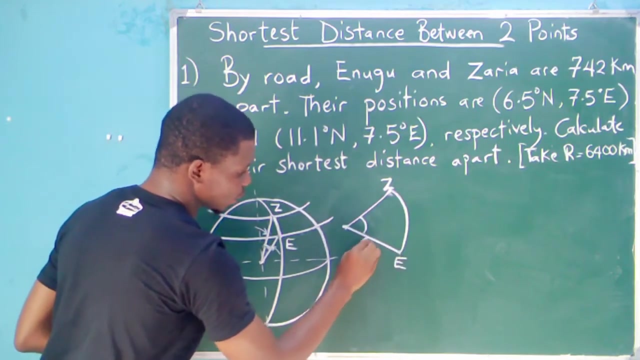 We have formed an arc. This is Zarya Z, This is Enugu. This point is this point, And then this one is this angle here, this angle here And then from here is the center of the Earth, here to this side, is the radius of the Earth. 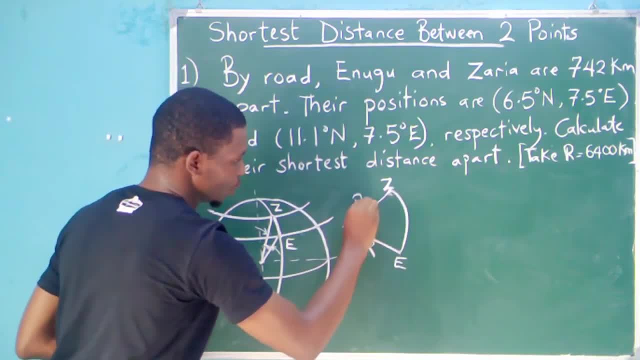 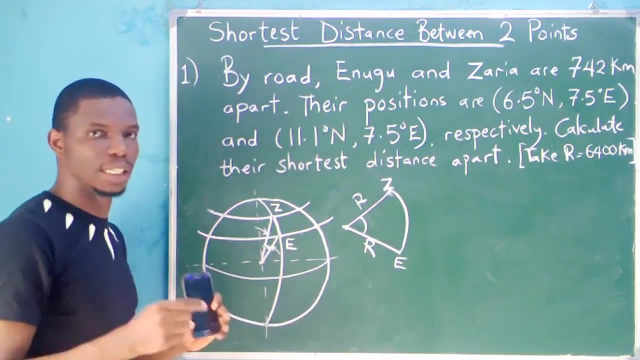 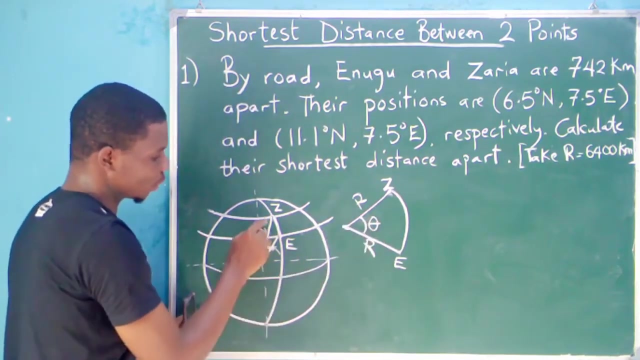 This one too, from here to here, is also the radius of the Earth. So now it becomes easy for us to calculate what ZE will be, because that is the length of an arc. Okay, And what would be this angle here? This angle, remember this one- is latitude 11 degrees. 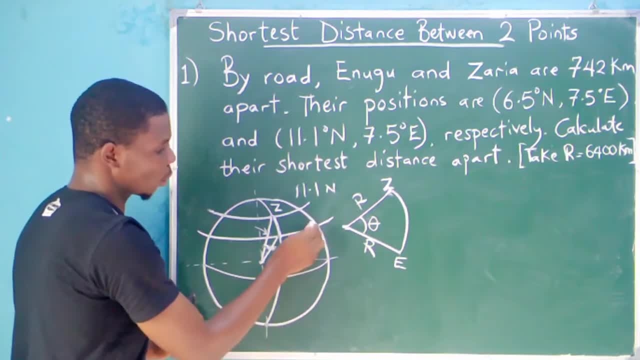 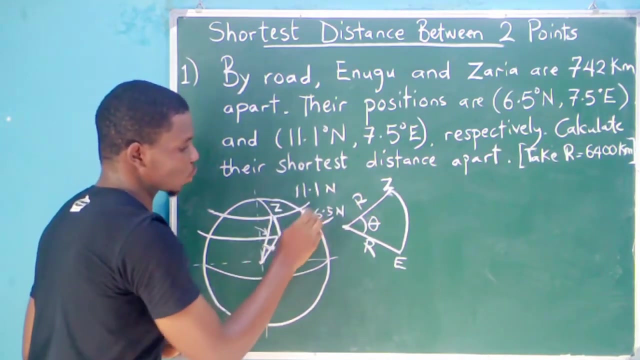 11.1 degrees north. right. Why this one is latitude: 6.5 degrees north, 6.5 degrees north. So what would be the angle between this and this? We just subtract 11.1 minus 6.5.. 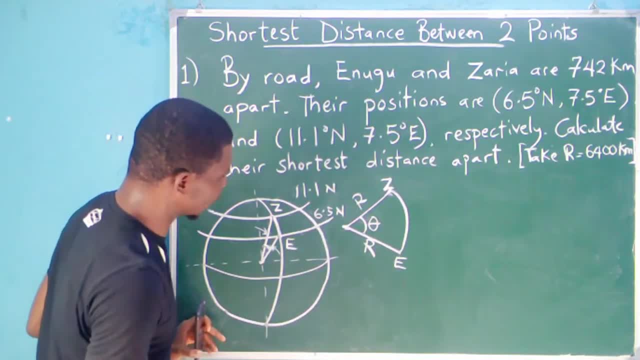 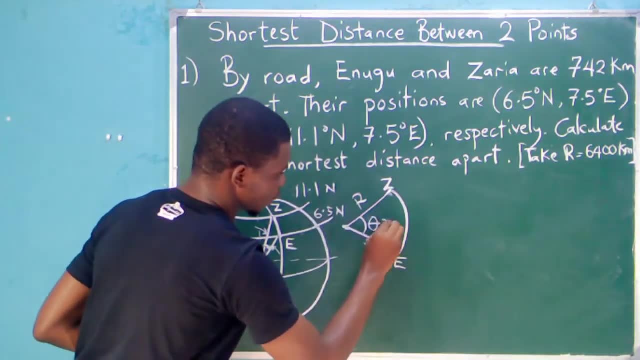 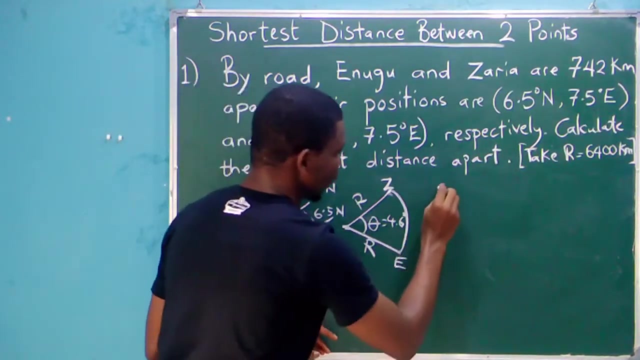 That is 4.6, right, Yes, 4.6.. So this is 4.6 degrees. So this angle is 4.6 degrees. So it's now easy for us to calculate ZE, which is the length of the arc. 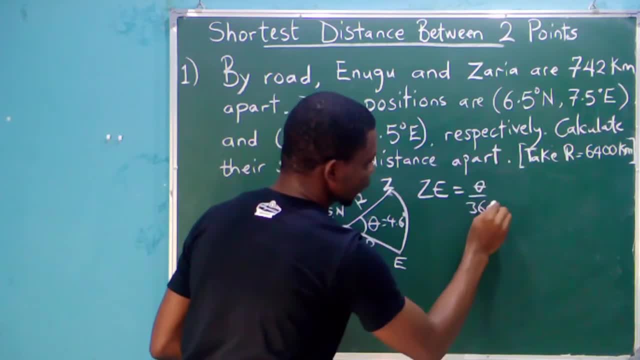 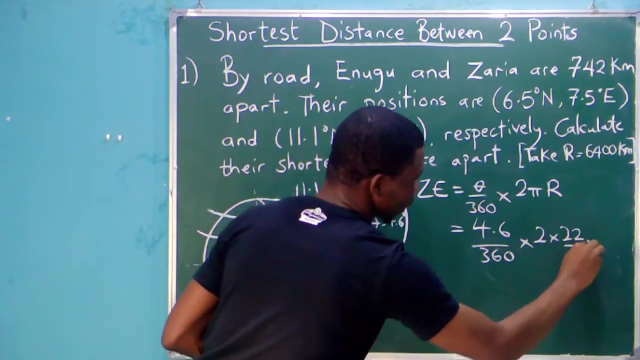 is theta over 360 times 2 pi r, And theta in this case is 4.6 over 360 times 2.. Pi is 27,, 22 over 7.. Then radius is 6400.. That is what we are given, the radius of the Earth. 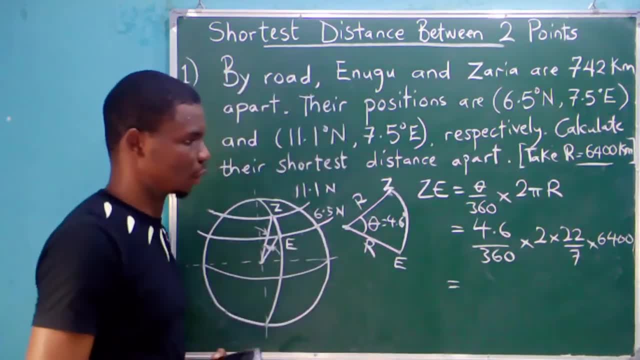 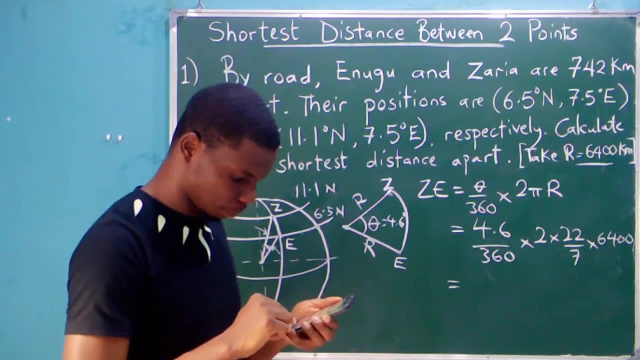 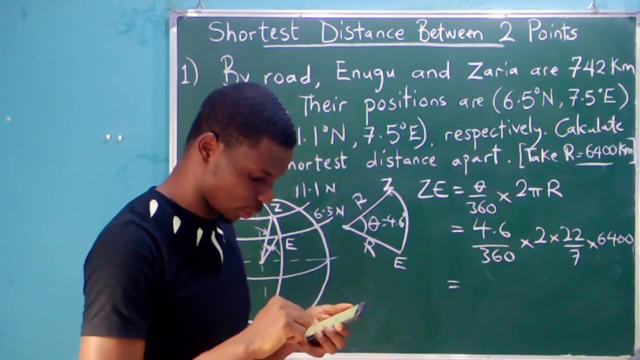 So you can now impute this in your calculator. Let me do it quickly. Let me get my calculator right. ZE is 4.6.. 4.6 divided 360 times 2 times 22 times 6400.. 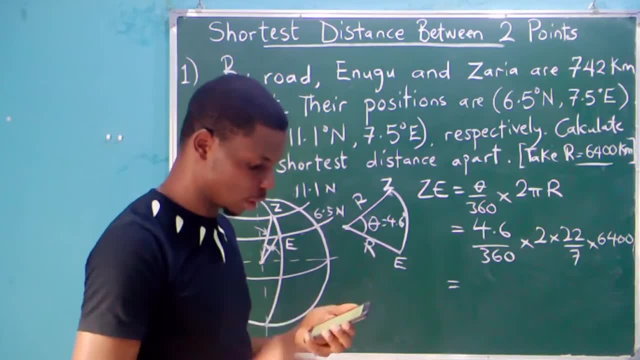 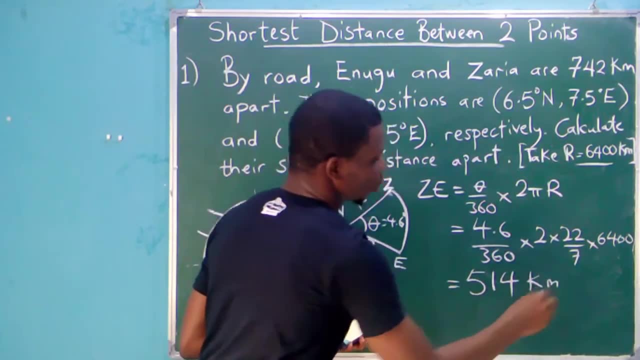 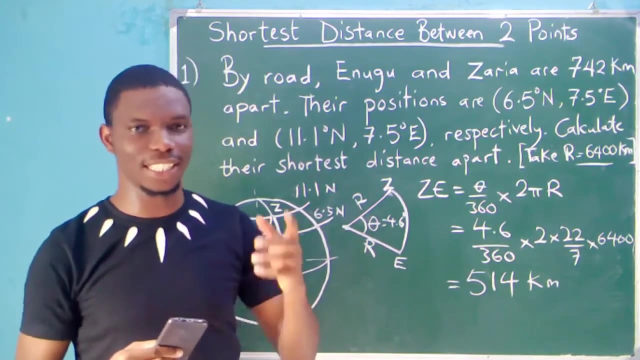 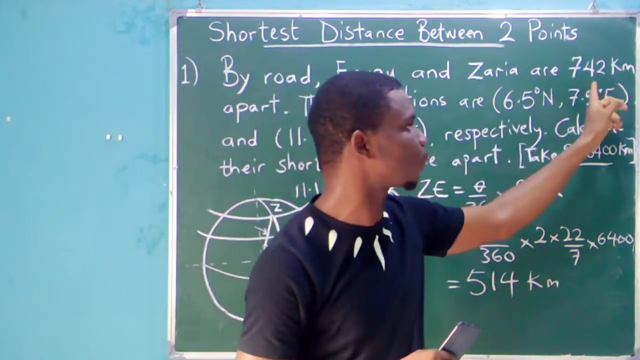 Then divide by 7.. So we have 514.. 514 kilometers. That would be the shortest distance between Enugu and Zaria. Alright, Now I said I have an interesting question for you. Remember they said: by road Enugu and Zaria is 742 kilometers. 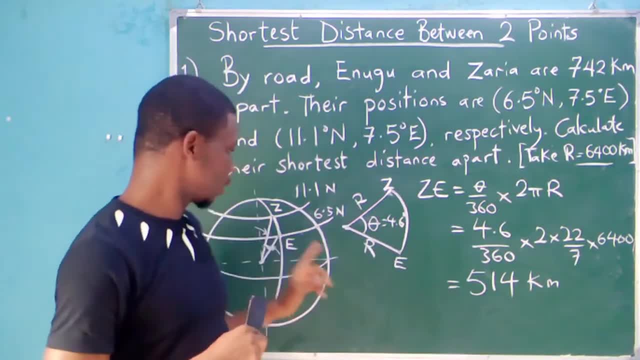 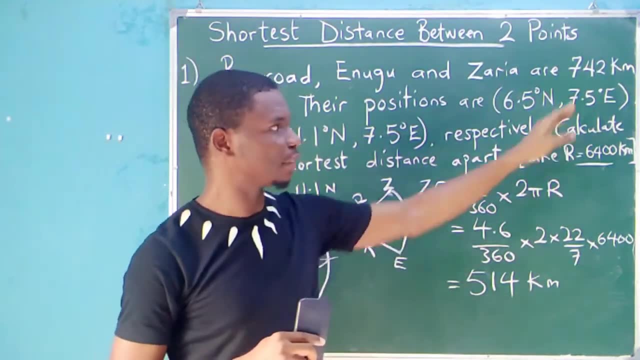 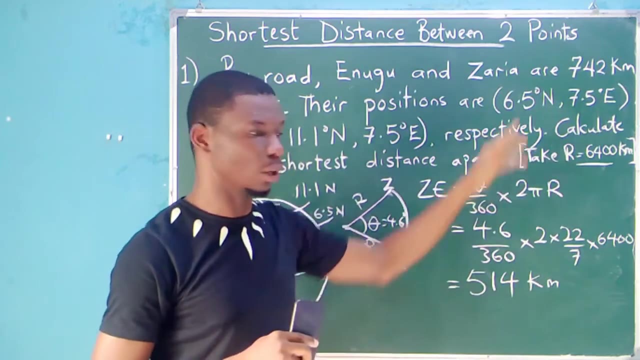 But now we have gotten the shortest distance between them, This from here to here, as 514.. Can you explain why? Why do we have this difference? Why is it different? Why is this one bigger, Farther than this one Or longer than this one? 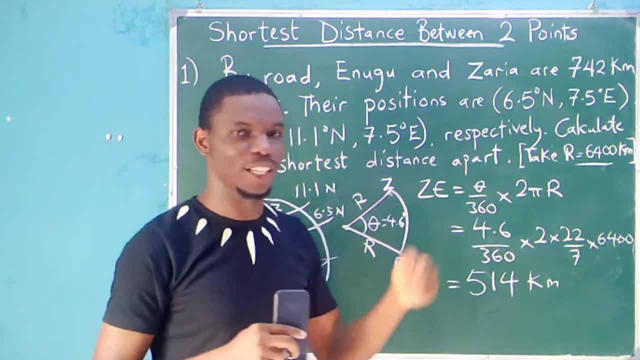 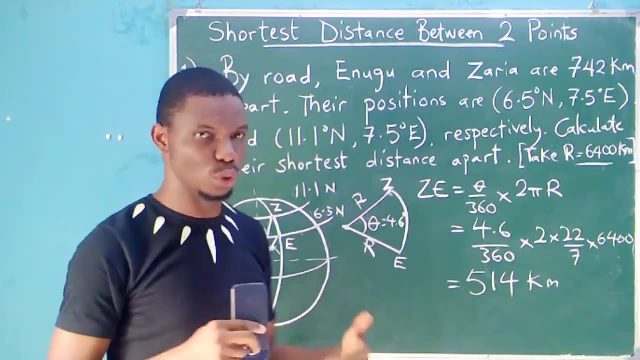 Okay, I would like you to put your answer in the comments, if you got it before, Because I am going to tell you why it is. But if you got the answer before I say it, I would like you to put it in the comments. 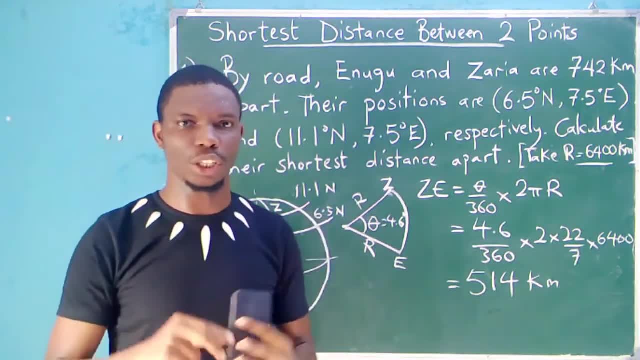 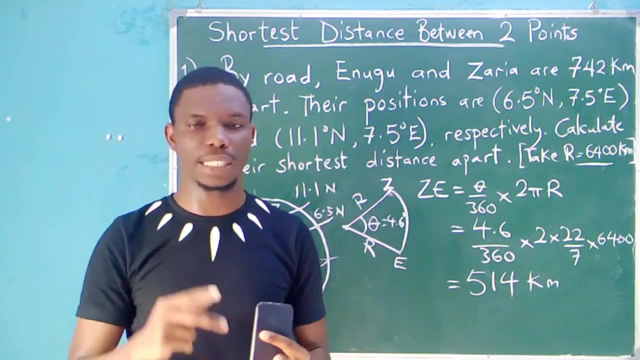 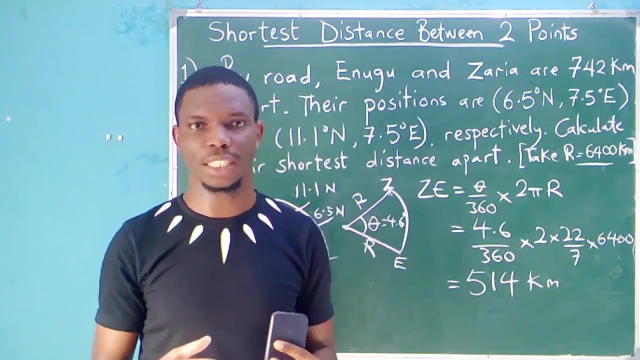 Now you know that the Earth is not just you know a perfect sphere like that. There are many. you know landforms, things like mountains, valleys, you know. And when engineers construct roads, they consider costs, you know. 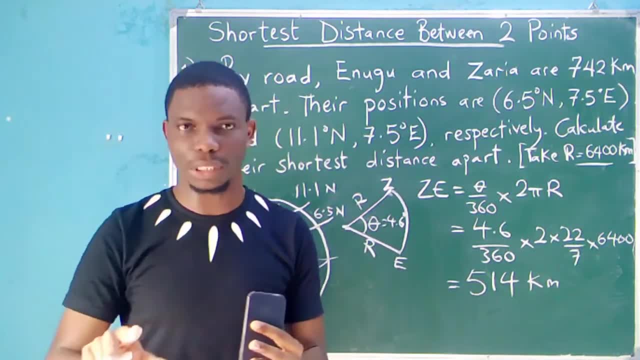 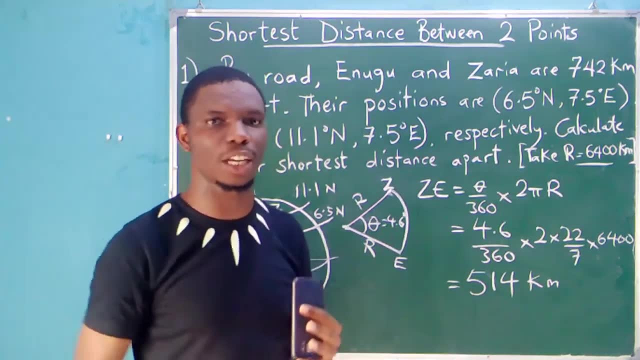 Is it economical to you know, try to break the mountains and make the road just straight that way. Or will it be more economical if they try to bypass that road, that mountain or that hill or that valley? Okay, What about rivers? 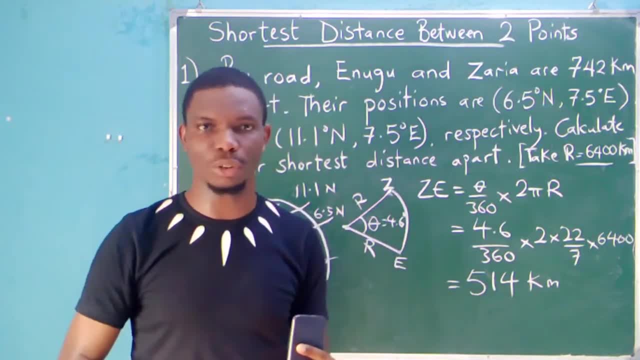 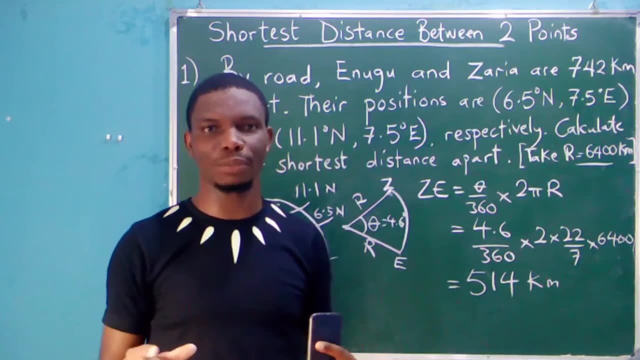 Will it be economical to build, you know- a bridge on top of the river, Or will it be more economical to go, you know, around it? So, considering all of these things, you can see that the road extension, the length of the road, will be getting longer and longer. 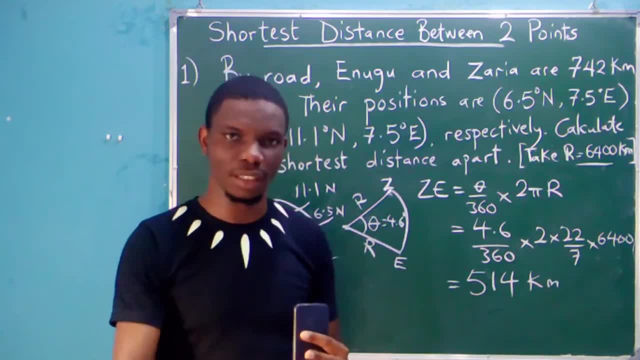 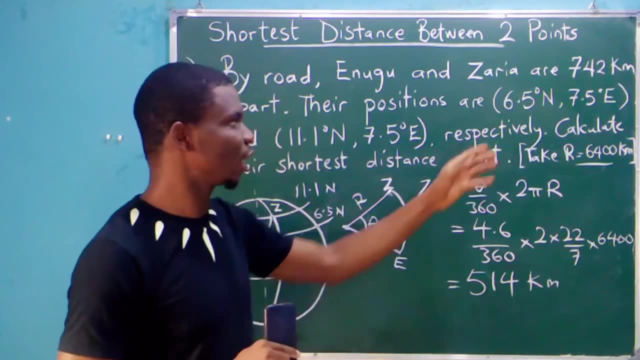 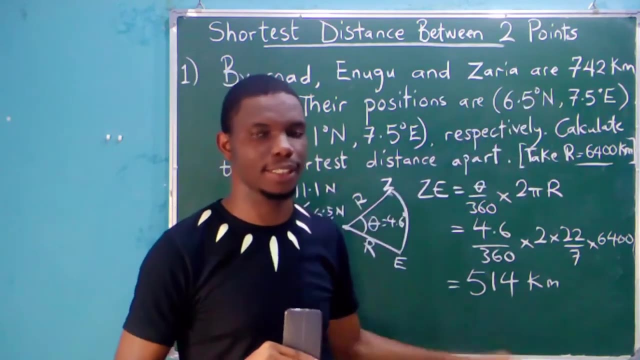 because you will be having curves, trying to negotiate the landforms, like mountains, like rivers, seas and all of that. So that is why we will not have the shortest distance between the two points to be exactly. you know this. We will have it longer than this. 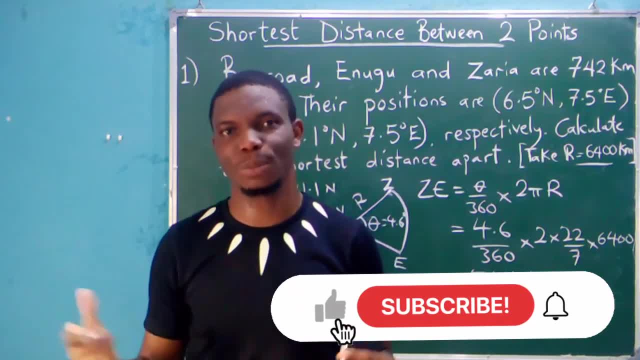 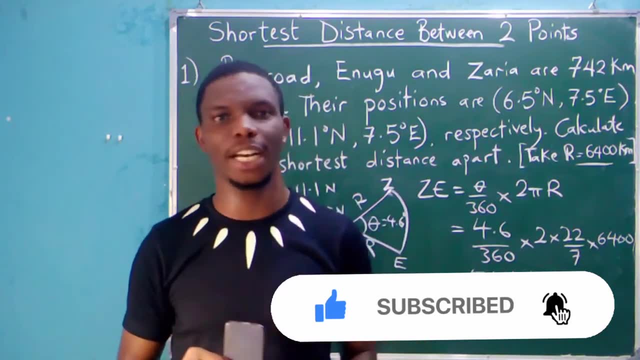 All right, If you enjoyed this video, why not like it? so YouTube can show this video to more people, And if you are new to this channel, consider subscribing. Click the bell icon so that you get notified whenever I upload new and interesting videos like this.